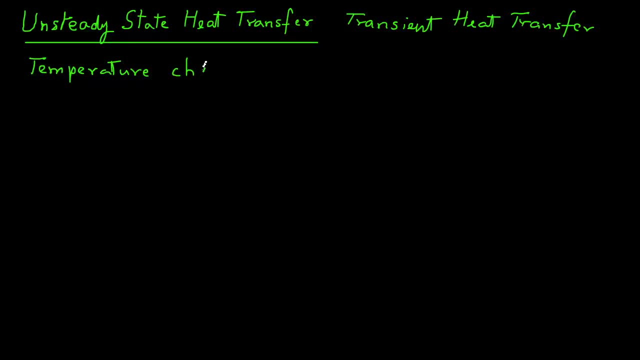 But now we will consider situations where, during heat transfer, the temperature in an object changes both with location and with time. Unsteady-state heat transfer is important in many food processing applications, such as in case of pasteurizing milk or in case of canning. 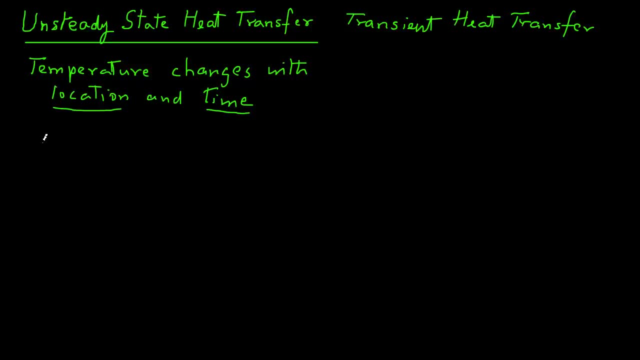 We will first look at the governing equation for transient heat transfer. This governing equation is a partial differential equation. We will not be solving this equation, We just want to get a better understanding of it. We want to get an understanding of how we can describe the change in temperature with time and location. 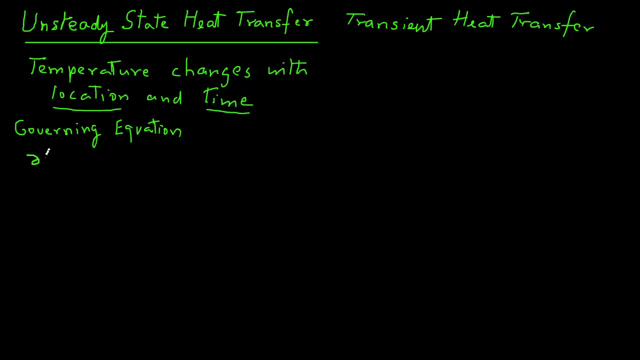 So the governing equation is partial T. this is upper case T for temperature divided by partial time, and we use the lower case T, for time equals K, where K is the thermal conductivity divided by rho, that is density, Cp, specific heat, r raised to power n and then partial over partial r and in parentheses we have r raised to power n. 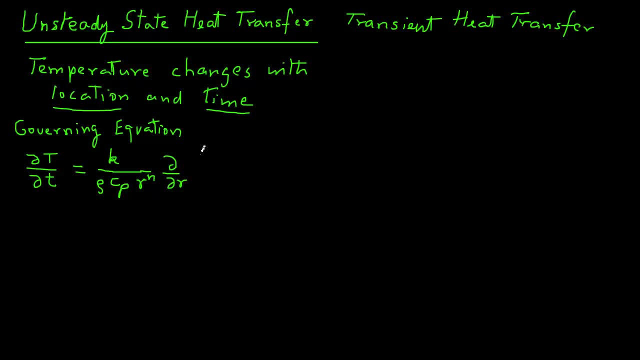 and partial T, that is, upper case T divided by partial r, and then close our parentheses Here. r is the distance from the center location of the object And n, which is the exponent, has three different values: n is equal to 0 for a slab shape, n is equal to 1 for a cylinder shape and it equals 2 for a sphere. 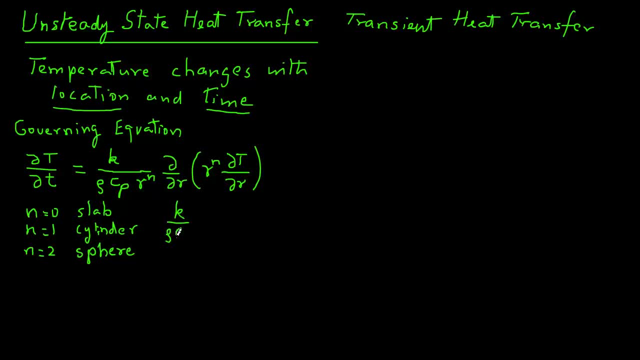 Note that the ratio K over rho Cp, which is essentially a combination of thermal properties, also equals the thermal diffusivity of the object, And thermal diffusivity we describe with a symbol, alpha. The solution of the partial differential equation is rather complicated. 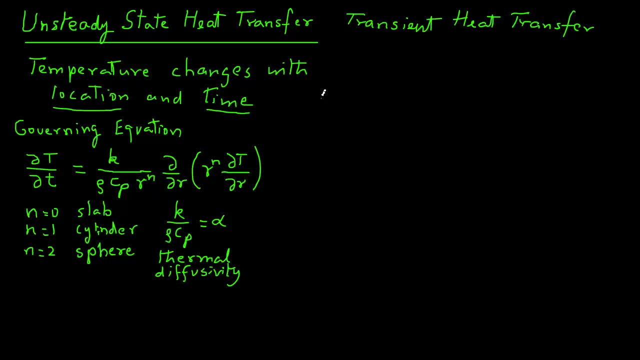 This equation can be solved only for three regular shapes, and those shapes are either for a very long cylinder, which we call infinite cylinder, or a very large slab, which we call an infinite slab or a sphere. Now let's see what we mean by a very long cylinder. 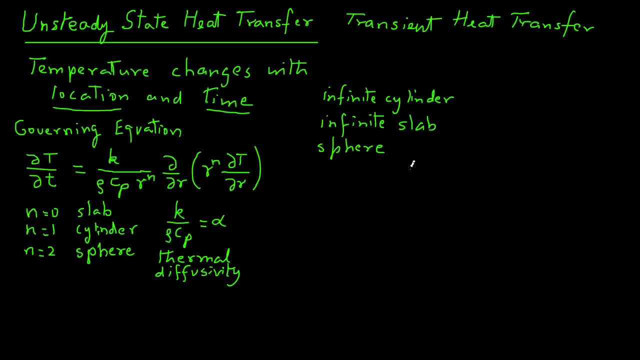 So here we have a cylindrical object, and we will consider that it is a very long cylinder, but it has a certain fixed radius. So the radius is r. Now let's assume that this cylindrical object is at a constant temperature, Ti. 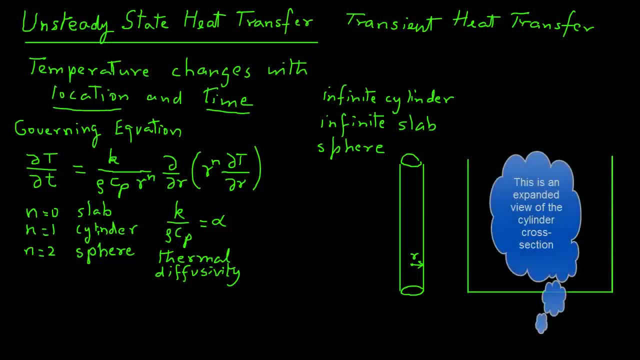 and we suddenly take this object and place it in a different environment where the temperature is much higher than the temperature of the object. Let's say that it is placed in a, perhaps in autoclave or some sort of an oven where the surrounding temperature is Ta. 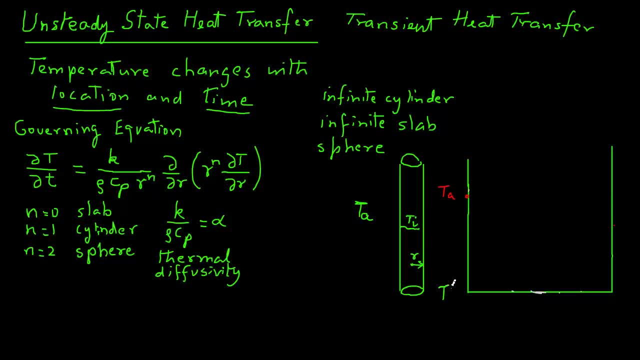 So your intuition will tell you that as the heat will transfer into this object, the surface will very quickly rise to the temperature of the surrounding environment, which is Ta. So we can show this here, that on both sides of this cylinder 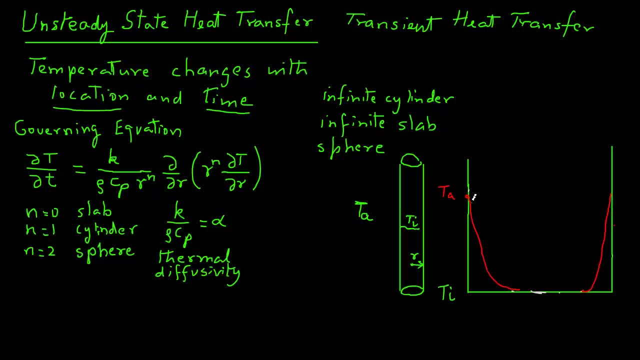 the temperature, in a very short period of time, will equal Ta, whereas in the center the temperature- since heat has not transferred to the center- the temperature will be still Ti. Now, if we leave this object in this heated environment, 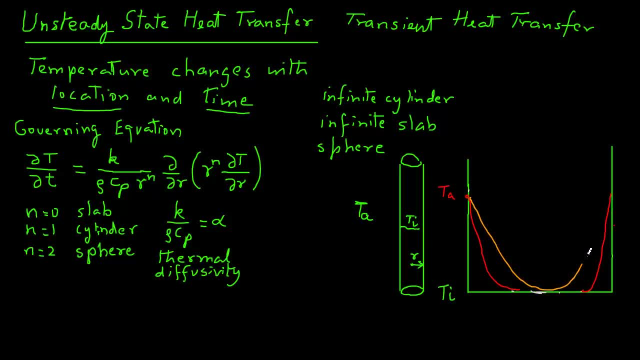 heat will be transferring into this object and after some period of time the temperature profile may look something like this, where now the temperature closer to the surface is increasing with time, but perhaps at the center it is still the same as the initial temperature. 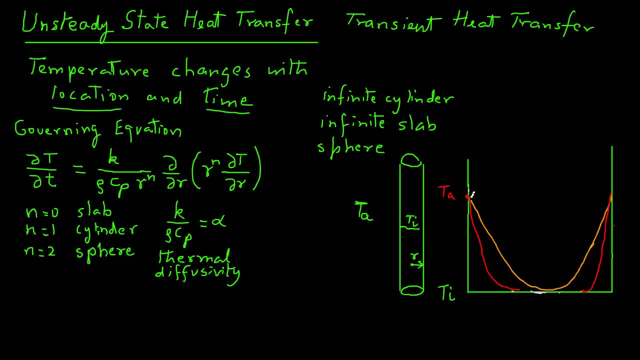 After we let it stay for a little bit longer, then more heat will transfer and at some point the center temperature will also begin to rise. And if you leave it for a sufficiently long period of time, the entire cross-section of that cylinder. 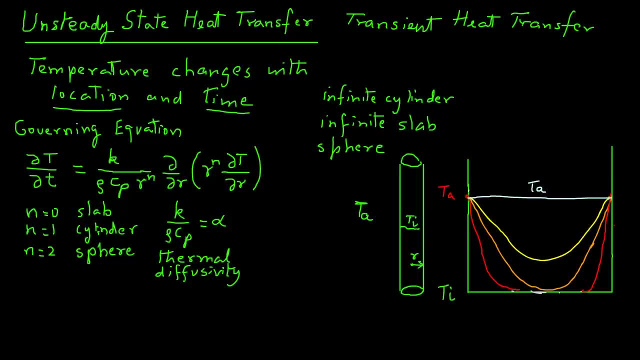 will reach the same temperature as the surrounding, which is Ta. So, as we see in this example, that as the heat was transferring from the surrounding to the center of this object, the temperature was changing with location and also it was changing with time. 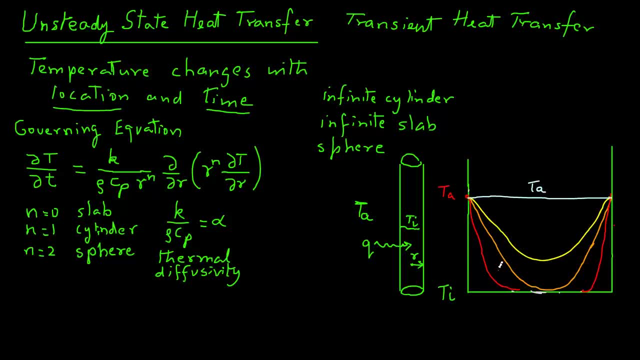 So we have this case of unsteady-state heat transfer, or transient heat transfer, into this cylindrical object. Now note that we did not consider any heat coming from the two ends of this cylindrical object, So we were assuming that there was no axial conduction. 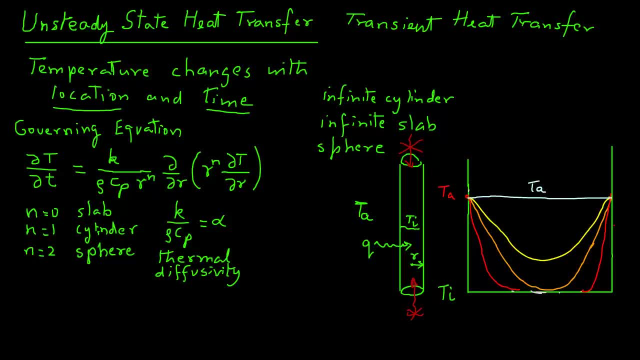 in other words, no heat transfer from the axis, but the heat was transferring only in the radial direction. This is the definition of an infinite cylinder, a case where there will be no heat transferring from the two ends of this cylindrical object, but heat will be transferring only in the radial direction. 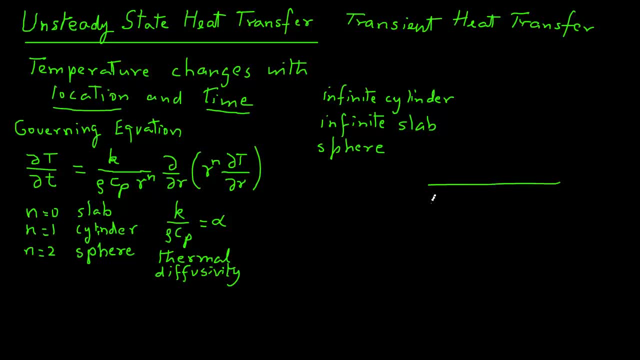 In a similar manner we can look at a very large plate or a slab, which we can call infinite slab, That has a fixed thickness. So let's say the thickness is 2Z, So the thickness of the slab all around is 2Z. 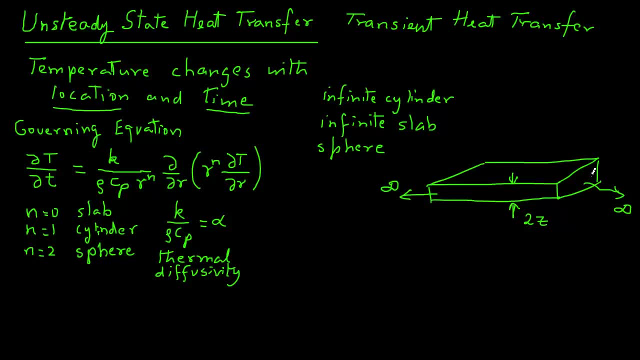 but it extends to infinity in all other directions. So when this slab-shaped object is placed in again in an autoclave or some oven, heat will be transferring from the top and the bottom side, but no heat will come from the sides of the object. 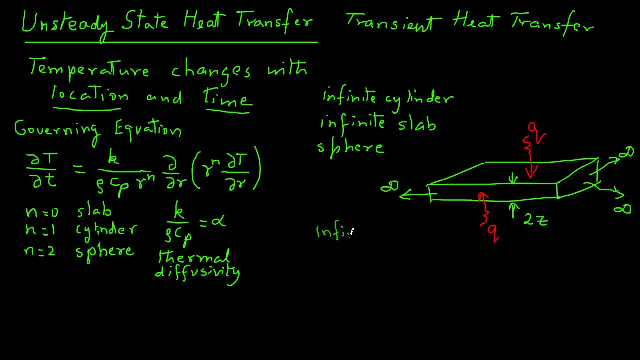 because the sides are too far off. So again, this will be a case of an infinite slab, where the infinite slab has one of the dimensions fixed, in this case 2Z, and all the other sides extend to infinity. And the third case is of a sphere.